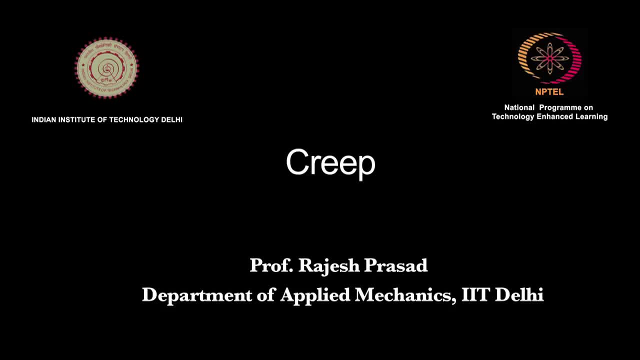 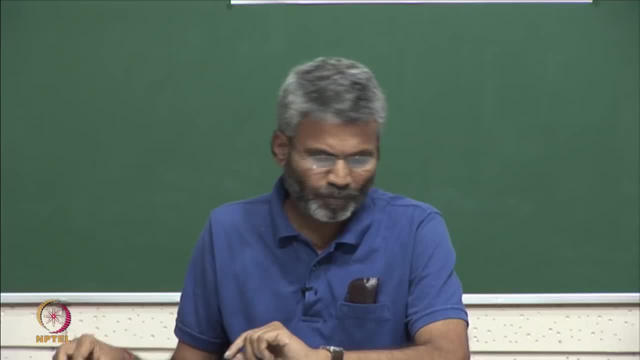 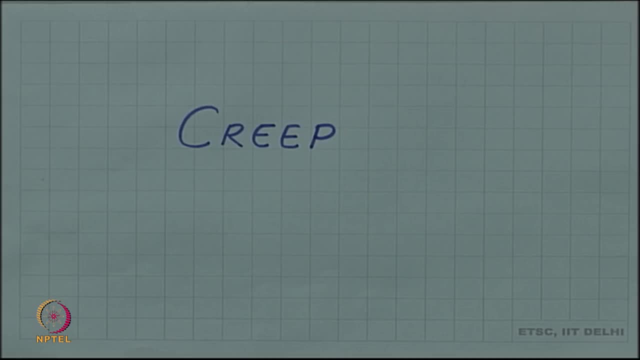 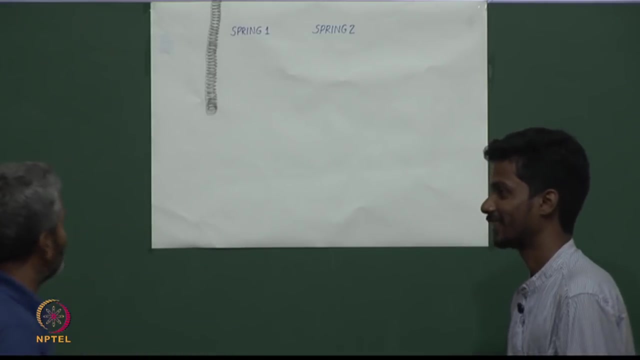 Today we are going to discuss a phenomenon called creep. It is a kind of a special kind of plastic deformation. but before we get into the detailed discussion of this phenomenon, let us look at a demonstration by Srikanth. Here is Srikanth, ready with his demo. What? 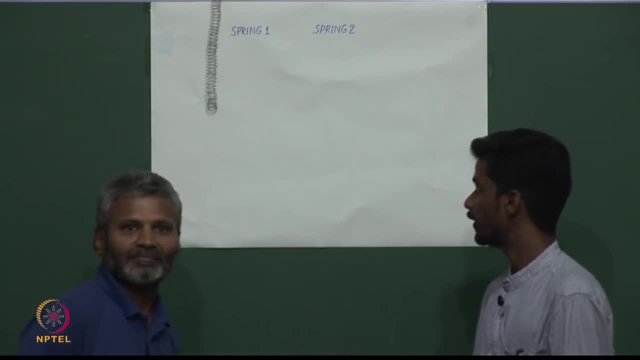 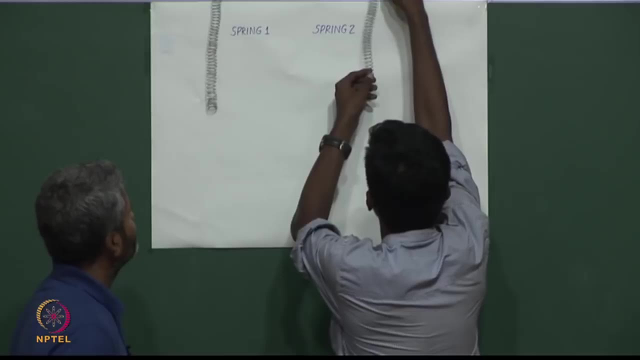 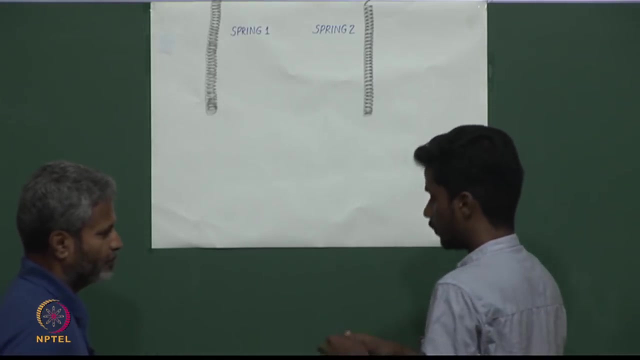 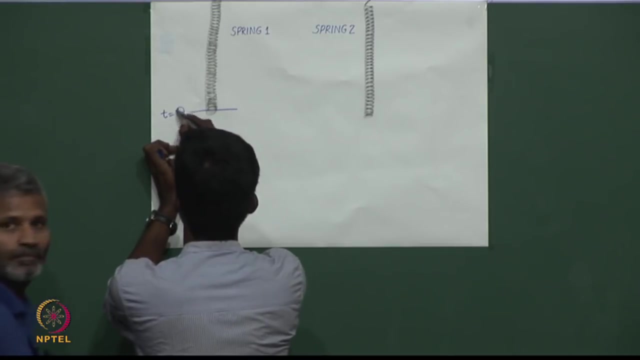 do you have Srikanth? I have two springs. One is already up there, The second one is with me. I will be putting it up And I will be marking the end points of both the springs and I will be marking the end points of both the springs. 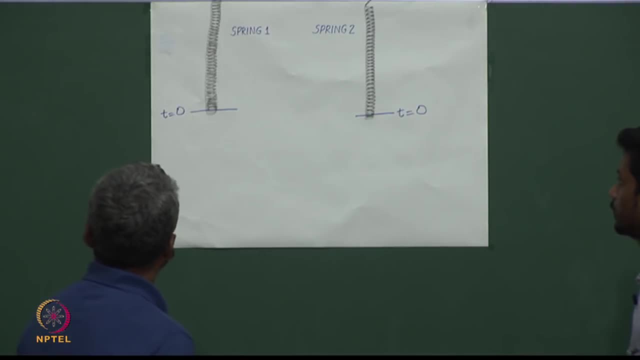 Okay, and I think you are going to put some weights on them. No, sir, I will not be putting any weights on them. We will just wait and see what happens. Oh, if you are not going to put any weight on them, what will happen? Nothing will happen. 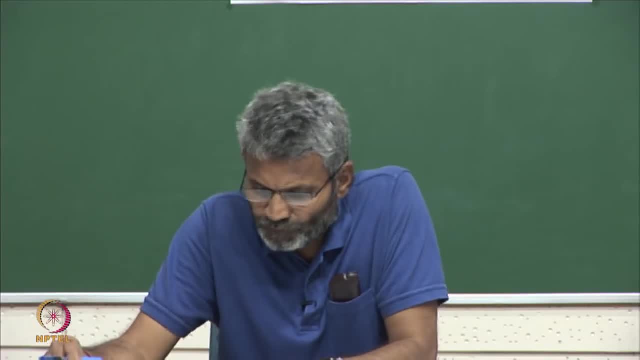 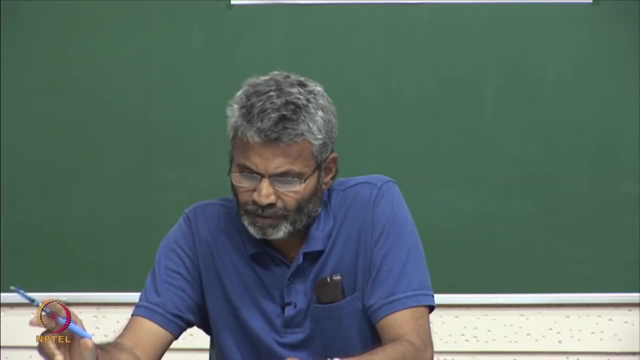 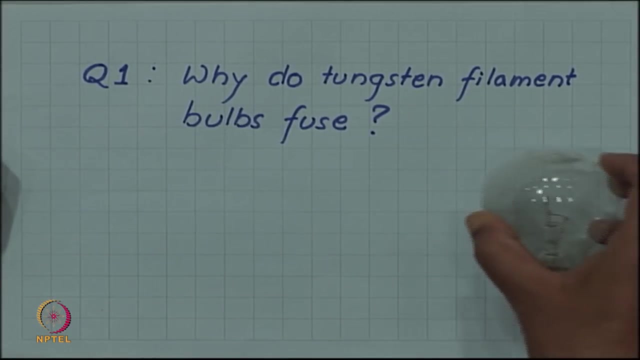 Let us see, sir, what happens While Srikanth's demo is going on. let us discuss some other interesting questions related to this phenomenon. The first question is: why do tungsten filament bulbs fuse? These are the over-otorphic. 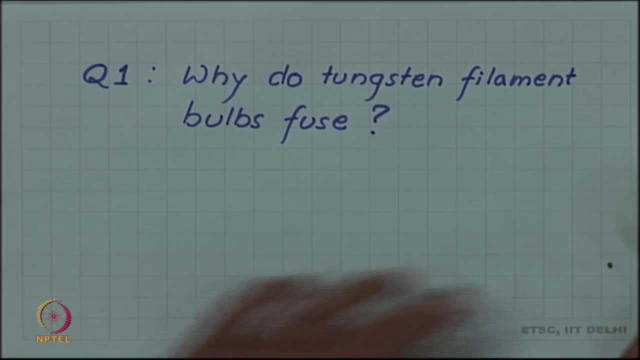 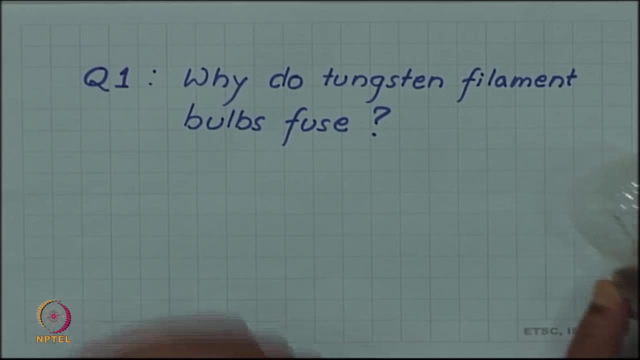 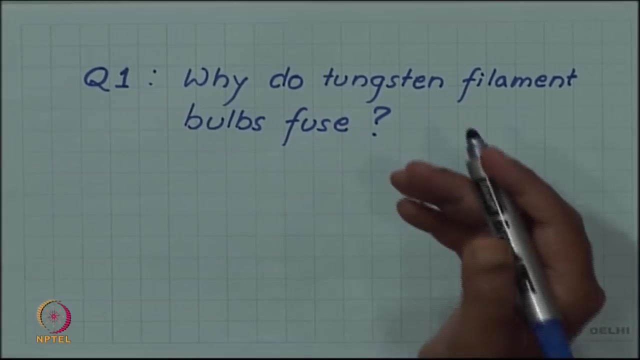 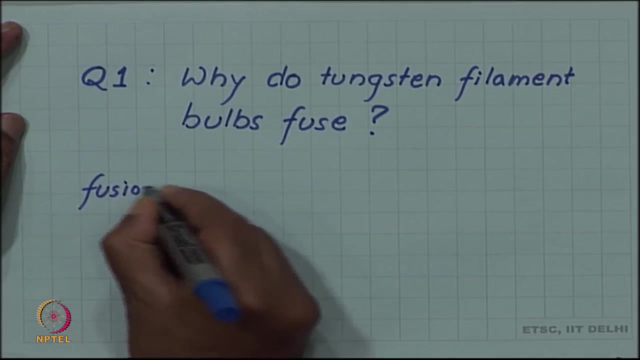 Okay, old fashion bulbs now going rapidly in obsolescence. you can see that there is a tungsten filament and that filament finally comes to an end of its life and that is called that. the bulb has fused. So why do bulb fuse? Now? fusion as such, the meaning of fusion, is melting. 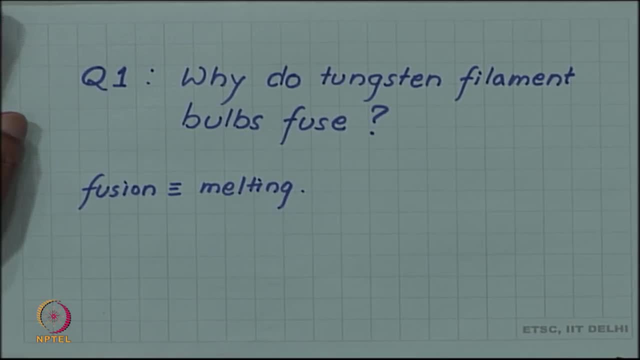 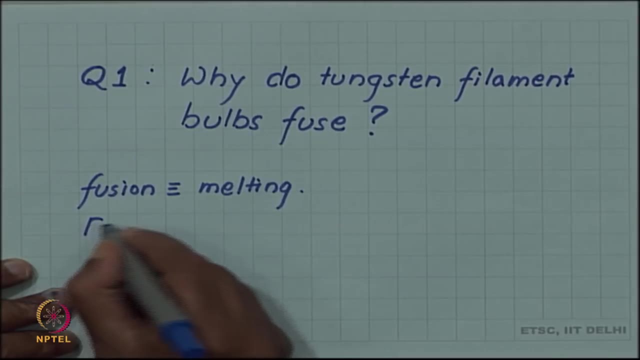 But does the bulb filament really melt? Filaments are made of. these filaments are made of tungsten and the melting point for tungsten is about 3410 degree Celsius. that is a very high temperature and if that sort of temperature can reach in the filament, that the not only filament- 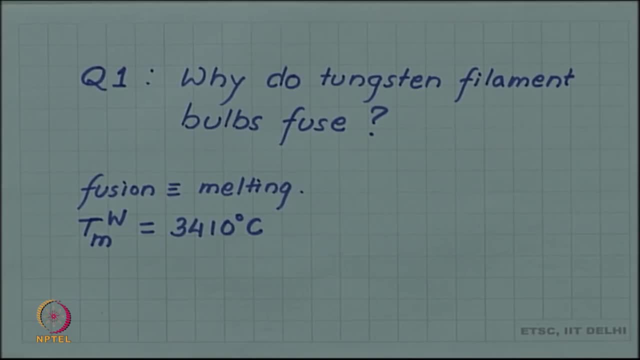 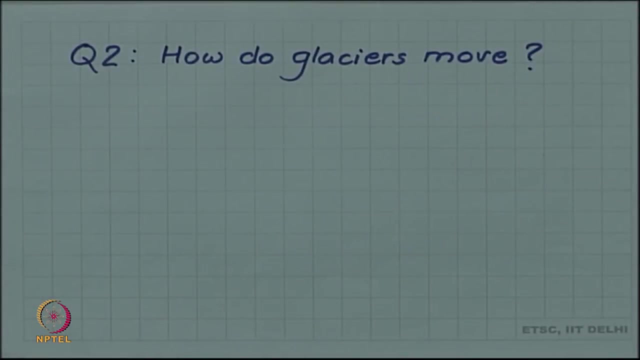 but many other components can also melt, but that does not happen. So may be the what we call bulb fusing or filament fusing is not really melting, but simply breaking. Another question- now we are taking this question from geology- that: how do glaciers move Glaciers? 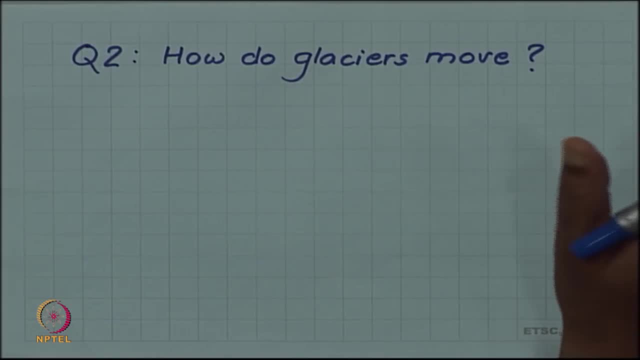 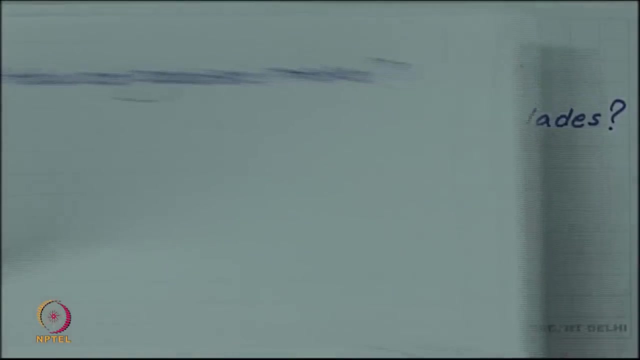 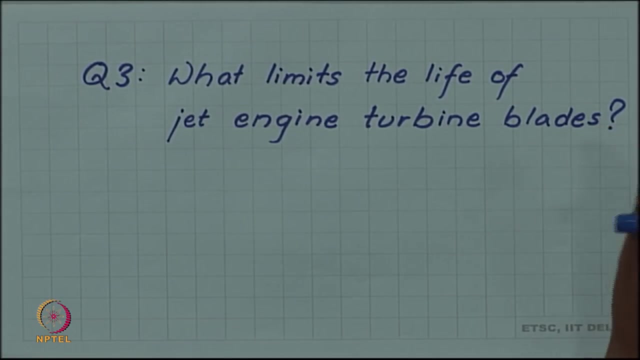 are huge mass of ice which are slowly moving. But is the movement just normal sliding or it is a deformation? We will look at that. And our final question is: what limits the life of jet engine turbine blades? I have some example of turbine blades from aircrafts of Indian air force you can see here. So 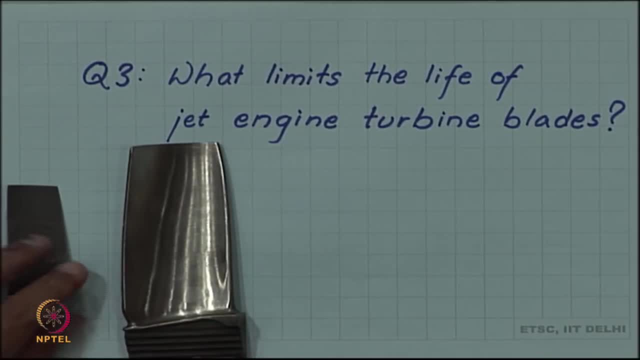 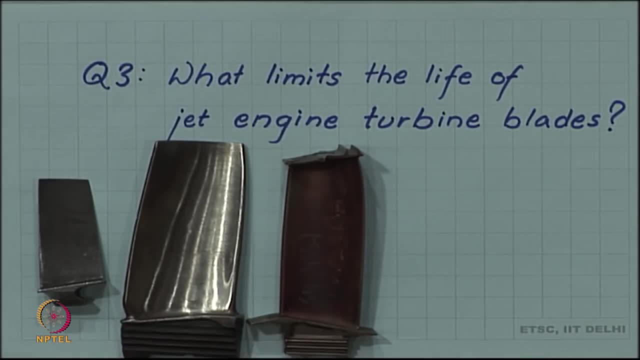 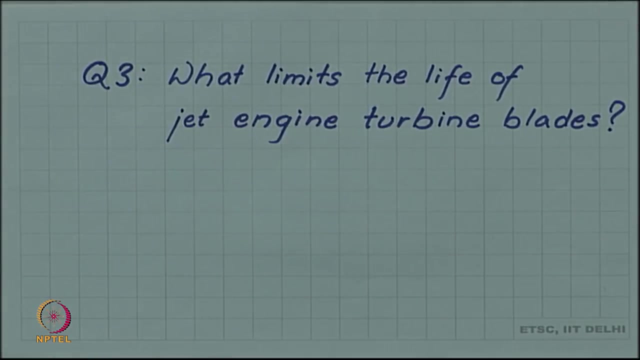 these are three turbine blades from different turbine of aircrafts. We will look at them in detail, but all of them have already failed and the failure involves certain deformation or certain deformation mechanism. What is that deformation? What causes the end of deformation, The end of a blades life? So these three questions are apparently related, apparently. 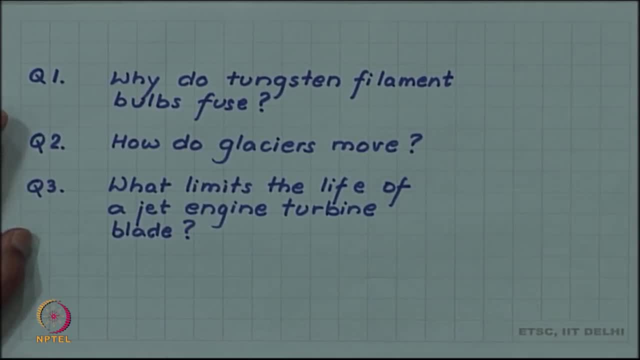 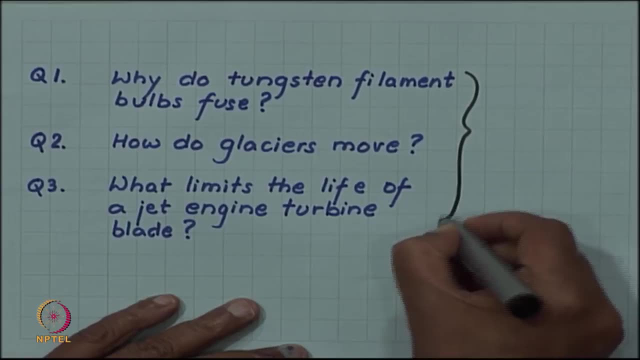 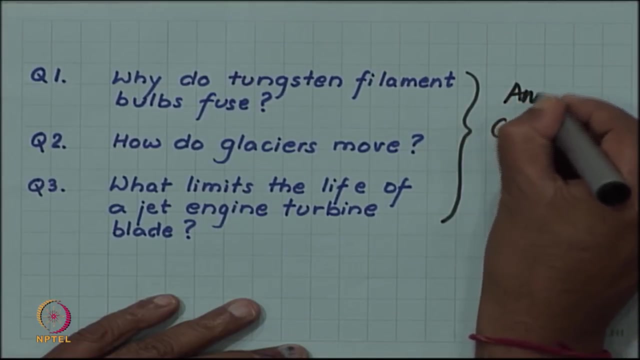 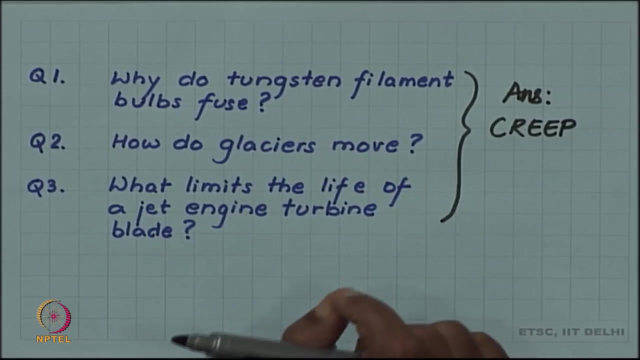 unrelated, but they are actually related because the answer to all these questions is the phenomenon which we are going to study, that is creep. So the tungsten filament bulbs fuse because the tungsten filament actually fails or breaks by creep. Glaciers move because it is not simple sliding of ice mass, but actually this: 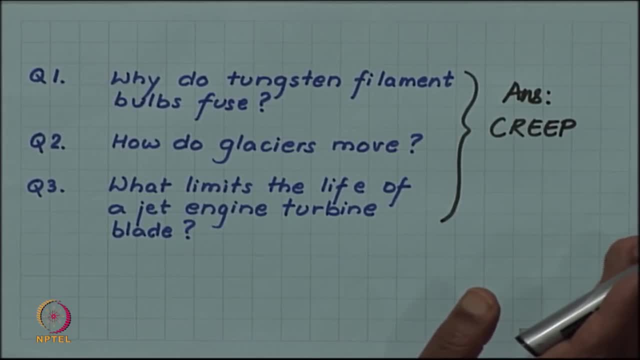 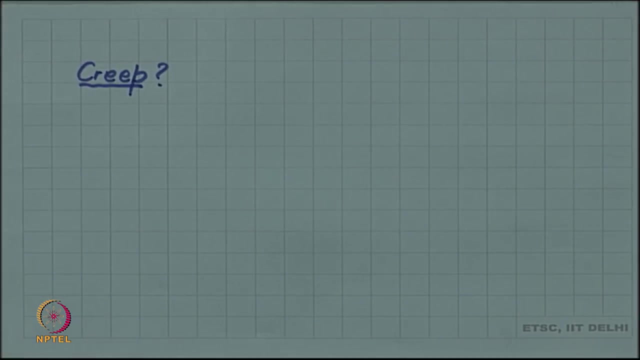 ice or snow deforms as the glaciers move, and the deformation mechanism is that of creep, And the limit of the life Of jet engine is also decided by the creeping of the blades. So then, what is this phenomenon of creep? So, before we answer this question, let us see how far our friend Srikanth has. 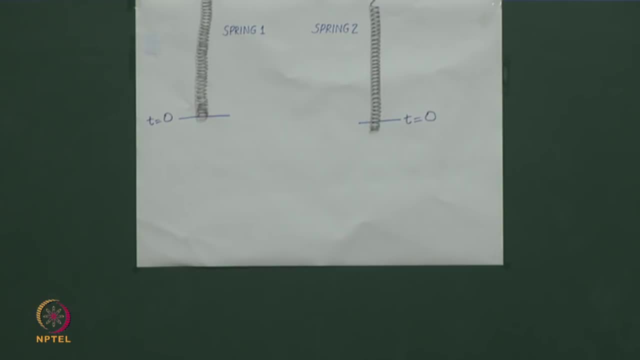 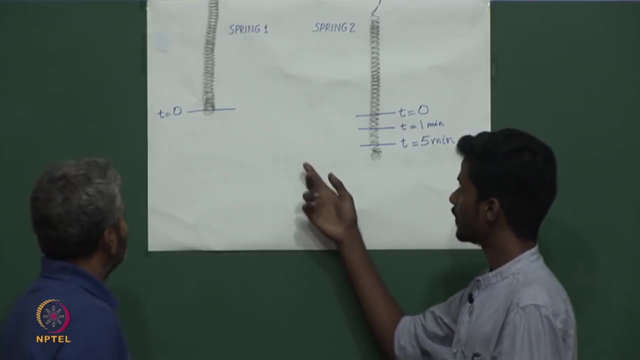 progressed. So let us start with the first question, And I have been noting down its end points after certain time intervals. 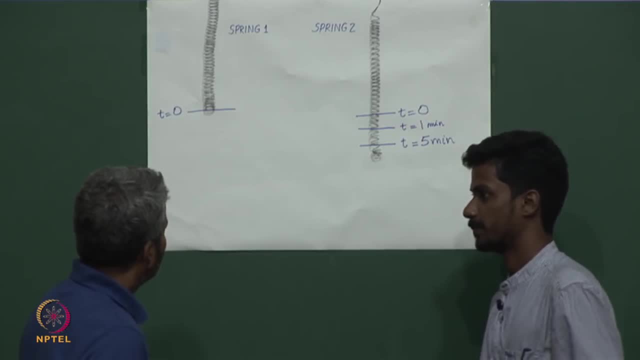 So I can see it is growing as a function of time without you increasing the load on it. There is some load on it- its own self weight- but beyond that you are not putting any load and that self weight is on this spring also. that is not elongating, of course, If I increase. 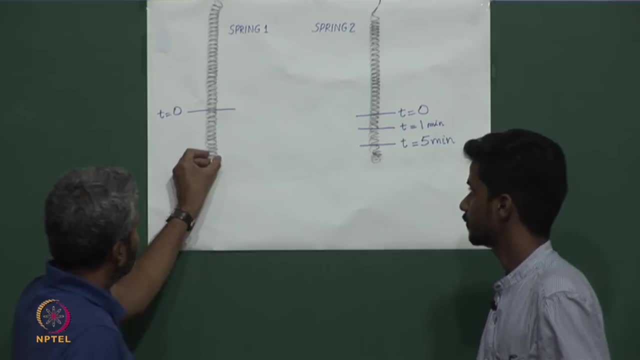 the force on it, I can elongate it. i can elongate it also, and this is elastic deformation. i think if i pull it hard enough it may undergo some plastic deformation also. so i have plastically deformed it, but for deformation i had to put an increasing load on it. but here 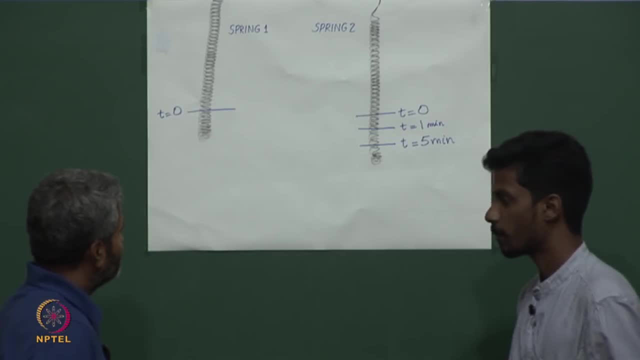 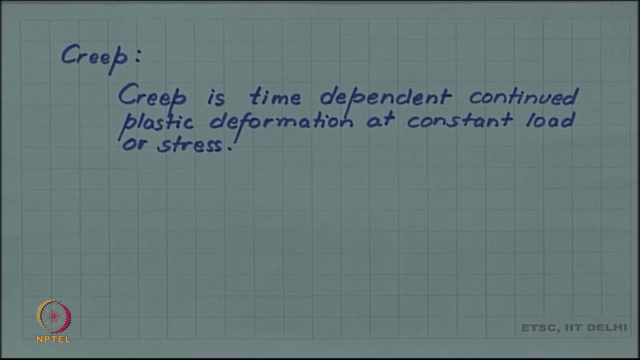 under constant load, the spring is deforming. yes, so this is a different kind of plastic deformation than the normal plastic deformation which spring one underwent when i put an extra load on it. so, as you saw in the case of that demo, that one of the springs was continually deforming, 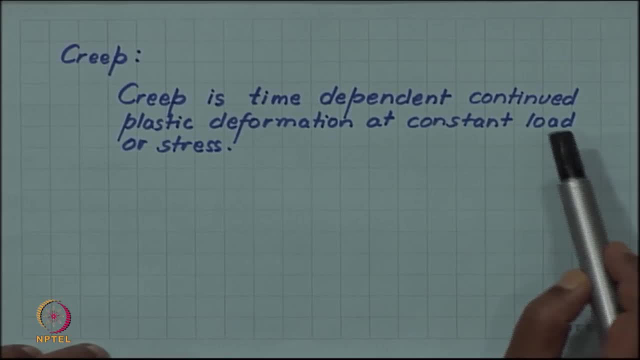 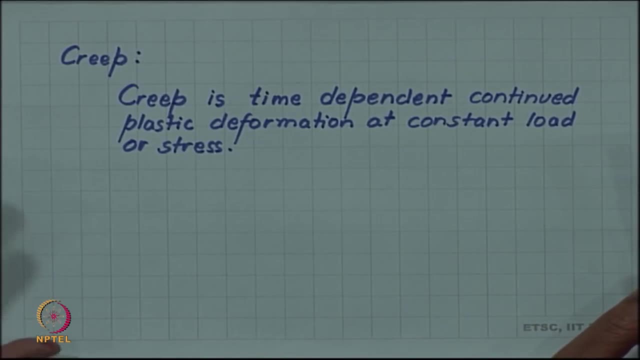 as a function of time. although we had put no load on it, although we had no not put any external load on it, its own self weight was still acting on it, but that self weight was constant. so under constant load, a spring two was continuously deforming. this kind of phenomenon is called 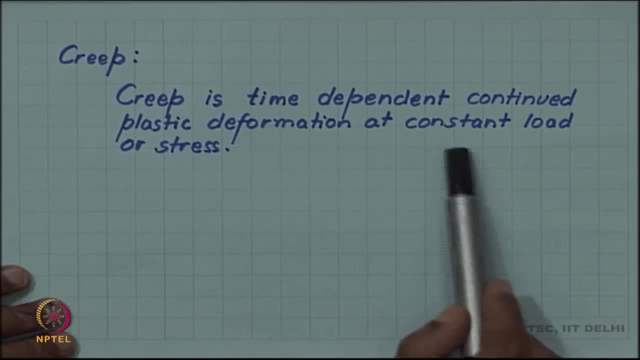 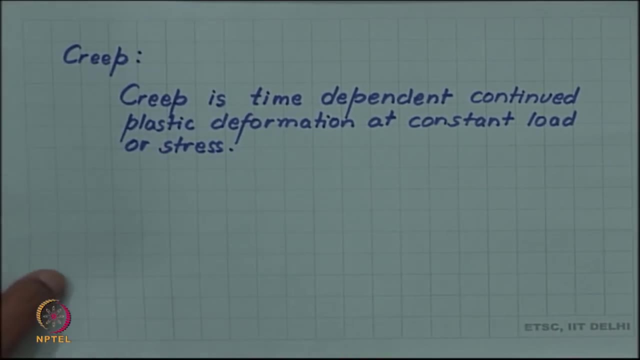 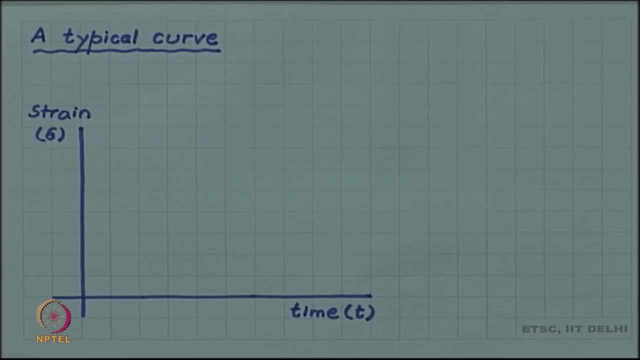 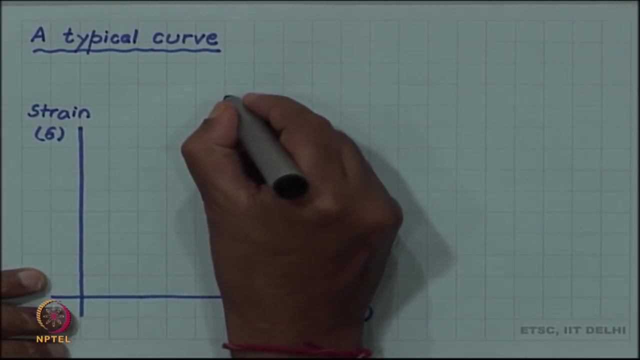 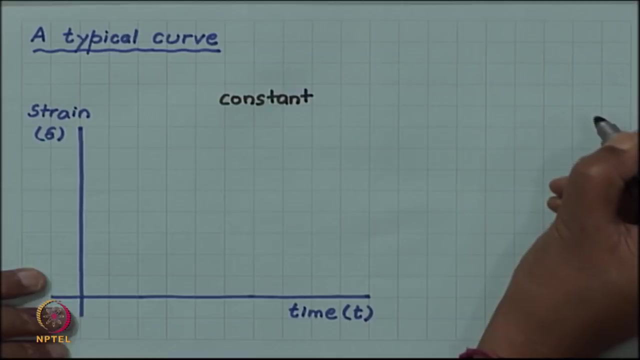 creep. so creep is time dependent: continued plastic deformation at constant load or constant stress. the results of creep test is usually plotted as a creep curve, where we plot strain as a function of time because we are keeping the stress constant and so, unlike the stress strain diagram which we had before, 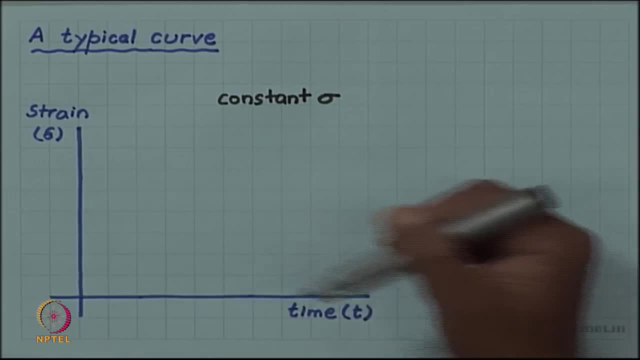 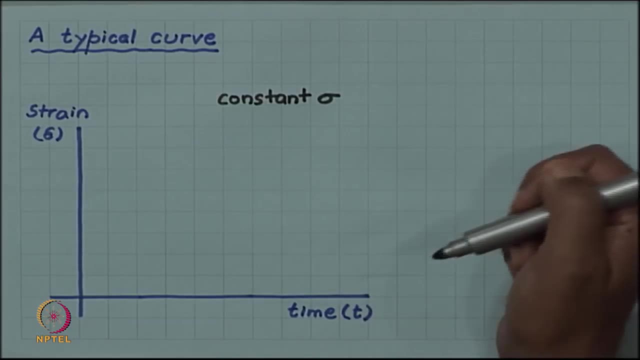 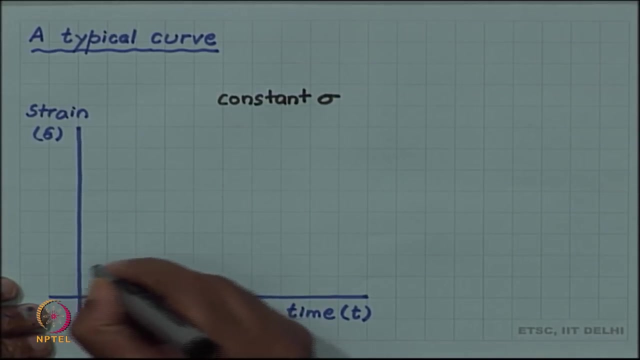 constant stress. we have a strain time diagram because it is a continued plastic deformation as a function of time. so a strain is plotted as a function of time. so if you plot a strain as a function of time you get what is called a creep curve. At time t is equal to 0, there 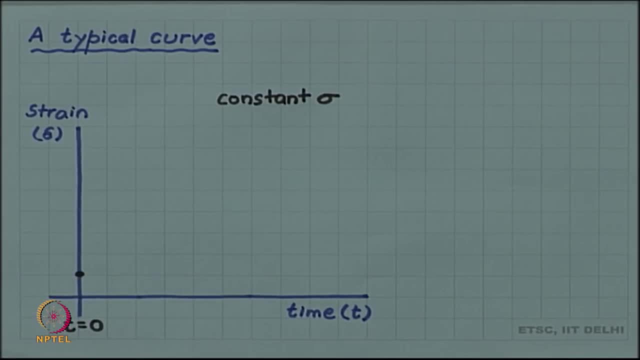 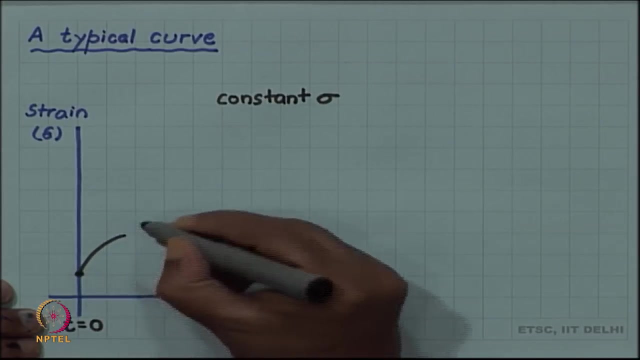 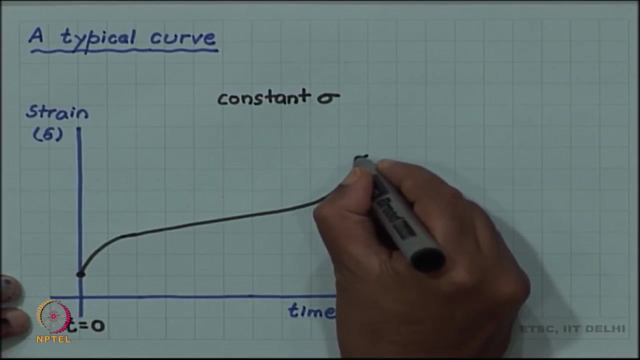 will be some initial deformation as soon as the load is put on the material. After that, even though load is not being increased as a function of time, material starts to deform and so the strain builds up And finally, at large enough strain, the material will break. 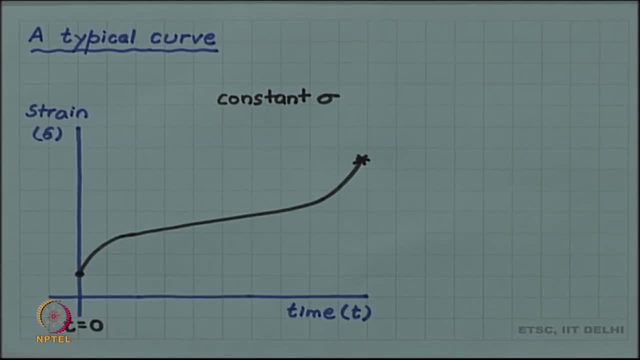 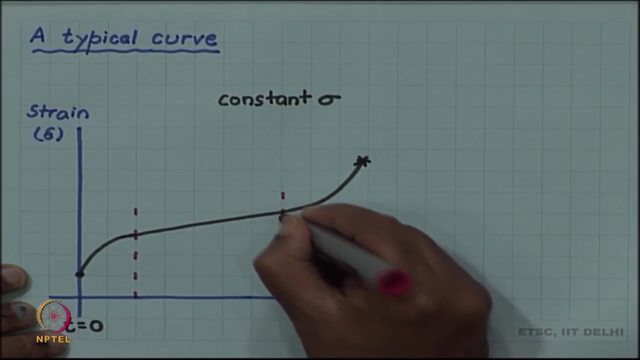 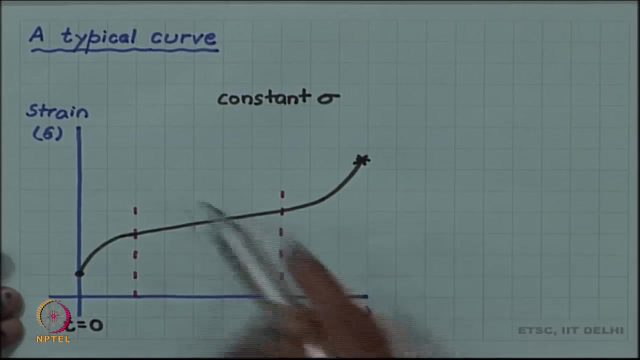 So you can see here That this is a typical creep curve of a strain as a function of time, with constant stress. Three stages are seen here. It is common to divide it in three stages: Stage 1, stage 2 and stage 3.. So let me write this. So the first stage is: 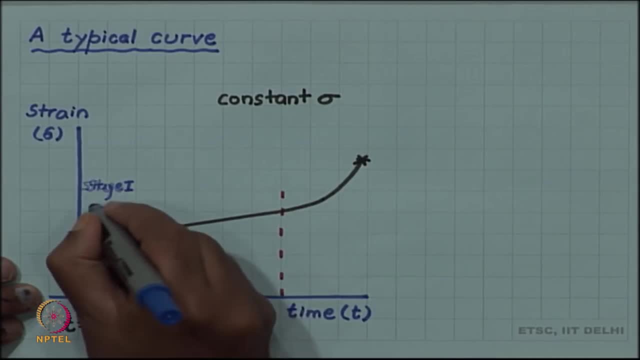 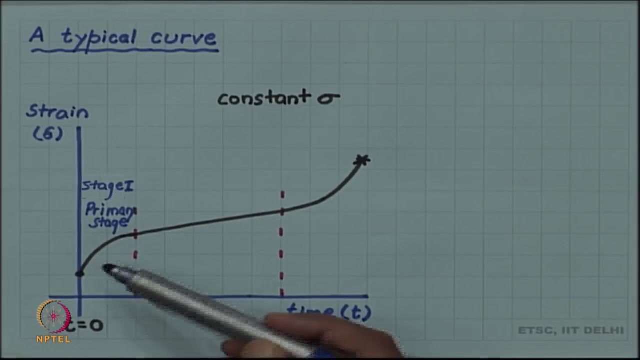 stage 1. It is also called primary stage. Here you can see that the creep rate was initially the strain rate of the creep curve is called the creep rate or the strain rate. So this strain rate is initially quite high and is gradually becoming less. So that is a stage. 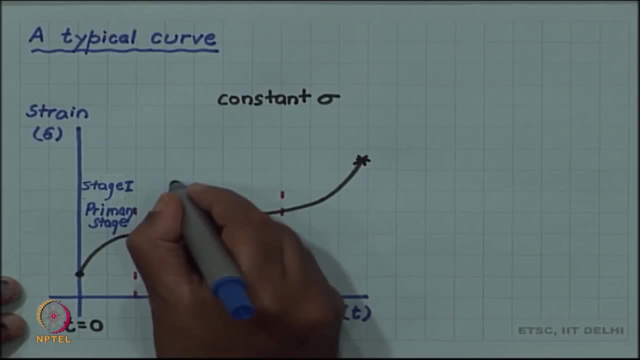 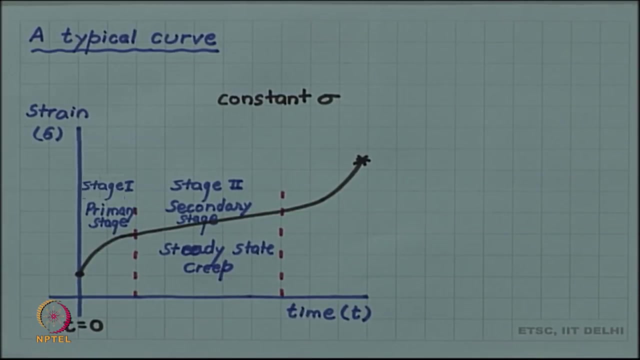 1.. Then we have a stage 2.. It is also called secondary creep or secondary stage, And this has one more name, because the creep rate is constant. This is also called steady state creep. And finally, at the end of the steady state creep, the creep rate again begins to. 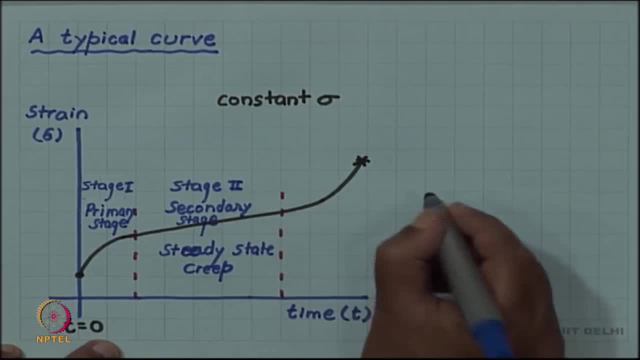 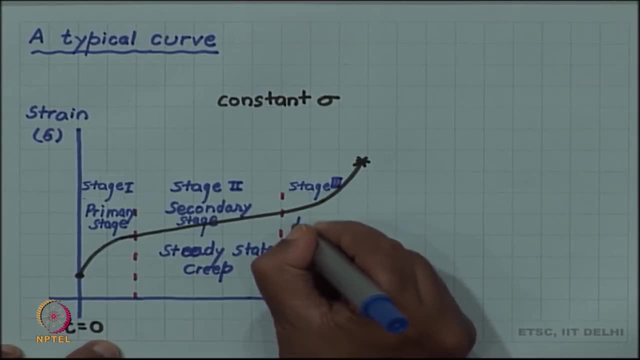 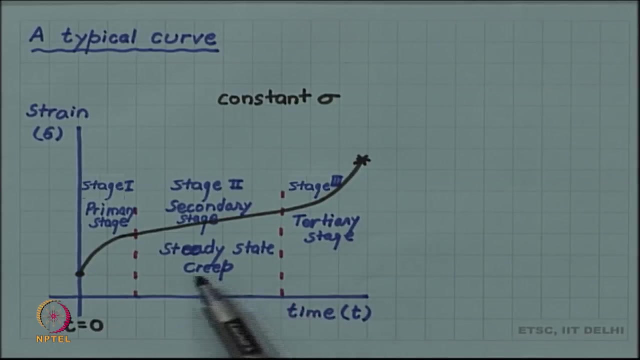 rise And finally leads to fracture. This is called a stage 3 or tertiary stage. So we have a stage 1, stage 2 and stage 3. Primary, secondary or tertiary. and the secondary stage also known as steady state creep, because the strain rate is constant. This constant is: 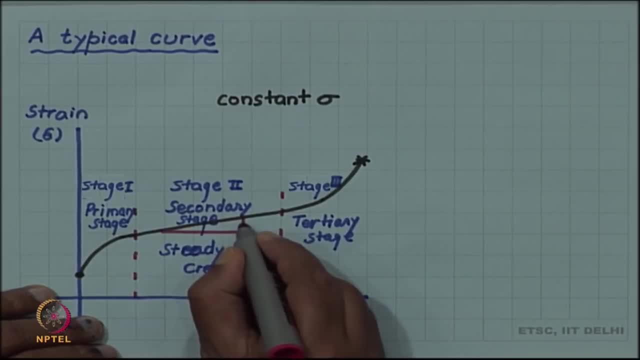 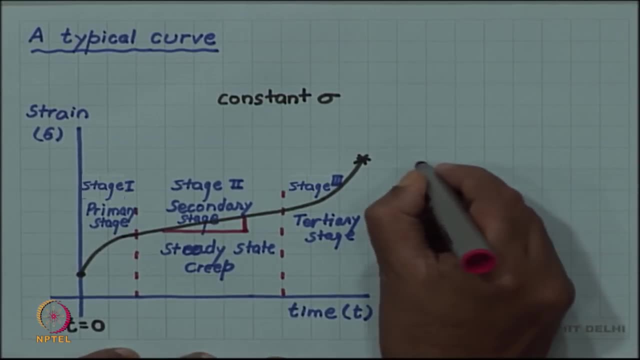 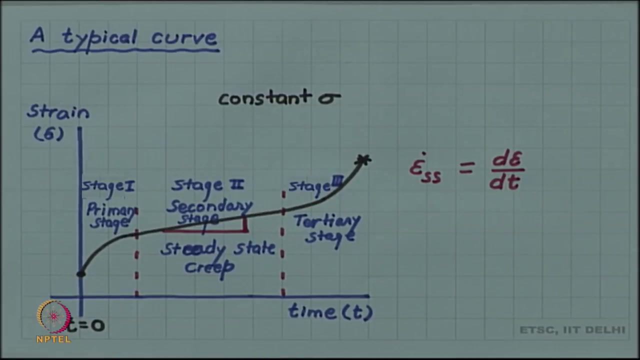 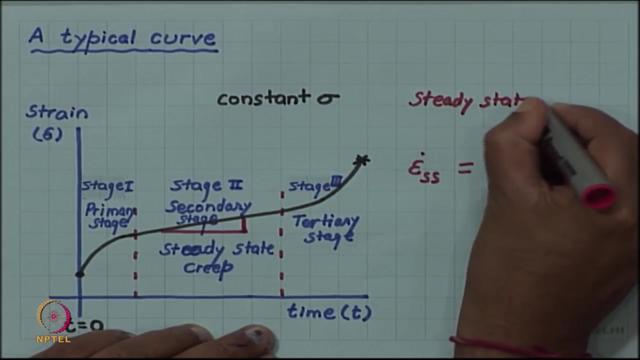 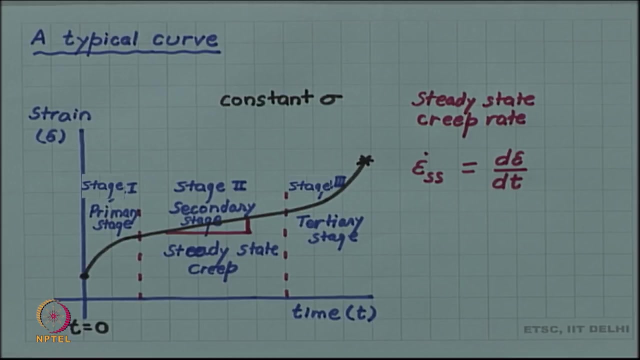 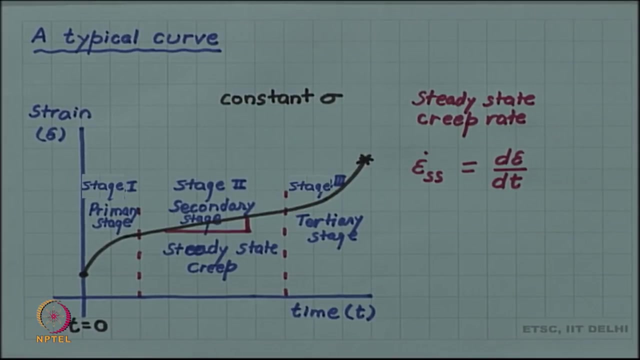 strain rate is important in the design of creep design or creep life of material, And this is called the steady state strain rate, which is the slope of the curve in the steady state regime. 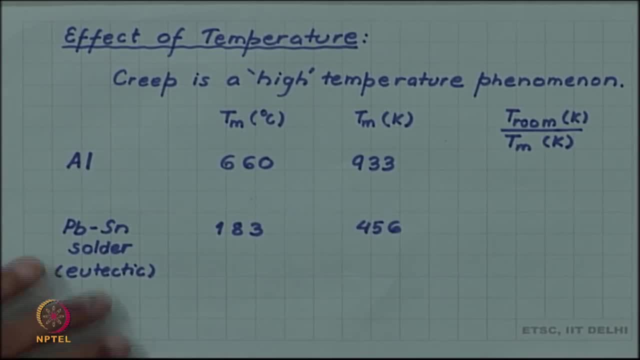 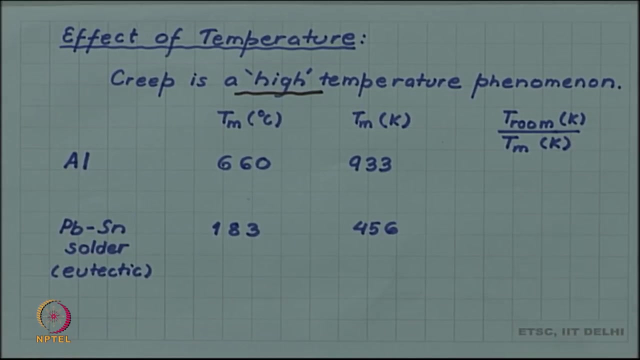 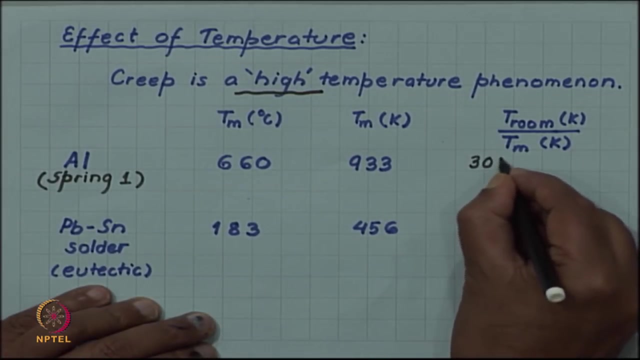 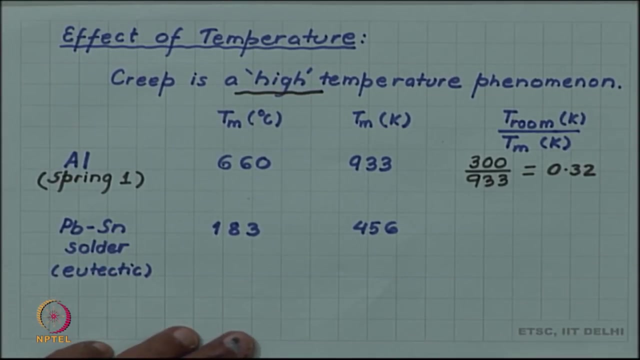 So you get a ratio of about 0.32, whereas for the let in solder wire, your spring 2 in the demo was let in solder wire. 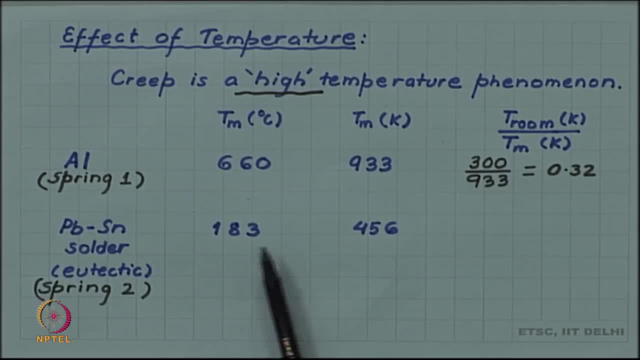 And as you remember from your phase diagram studies, that a eutectic solder has a melting point of 183 degree Celsius. So if you take that as the melting point and convert it into Kelvin, which is 456, then the same room temperature.